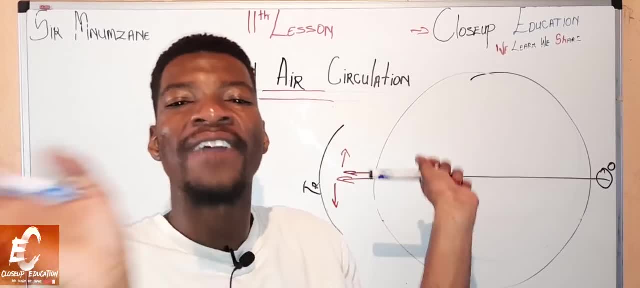 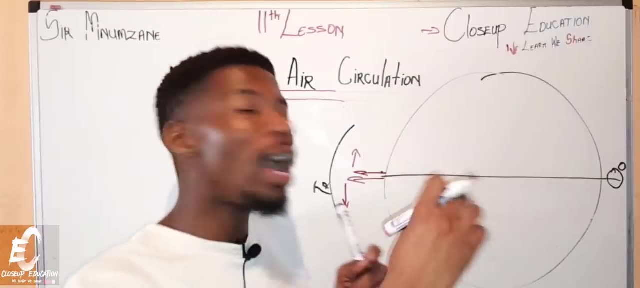 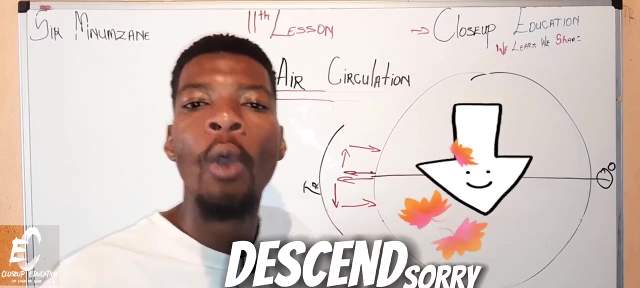 the tropopause right. and as the air diverges, it will obviously cool off, because of we know, the higher you go, the colder it gets. so, as the warm air cools, it will obviously ascend. this air will ascend and where is it ascending? it is ascending on a line which consists of: 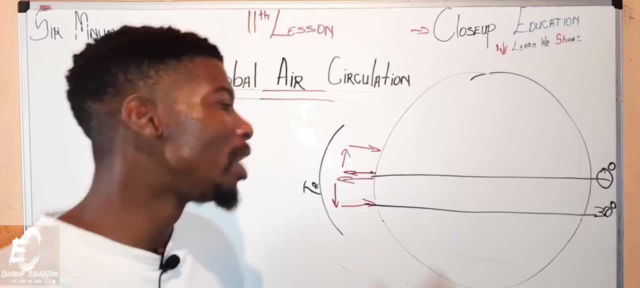 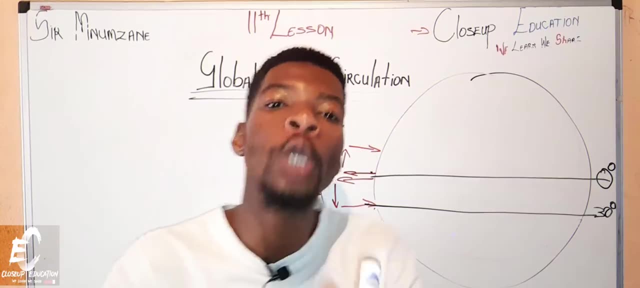 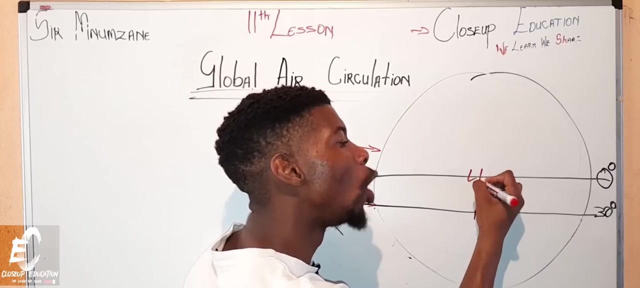 30 degrees Celsius. right, so we now know that the earth consists of 0 degrees. 30 degrees, then we have to continue. all right, but we know that the 30 degrees this means now we are on a high pressure. this was what a low pressure. now we are. 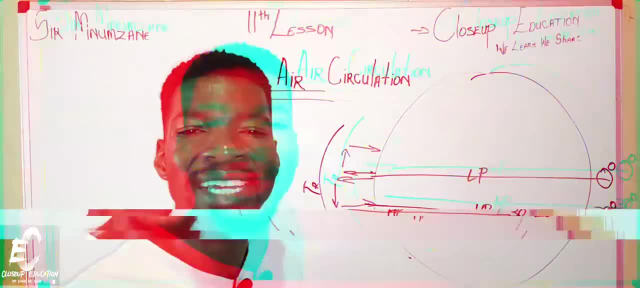 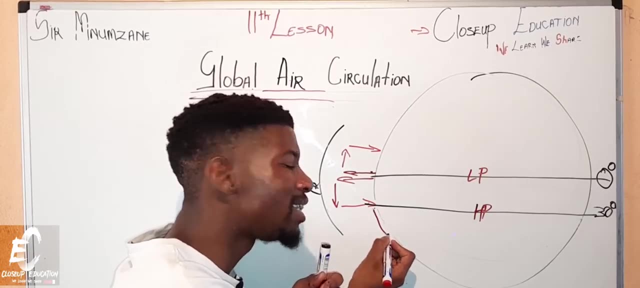 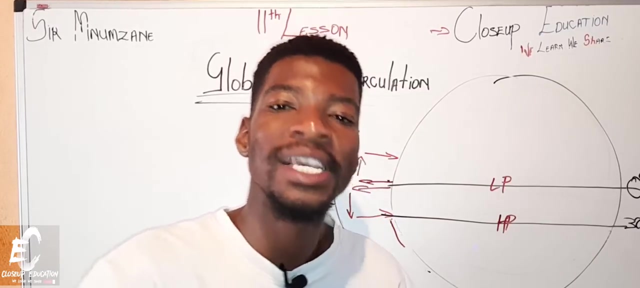 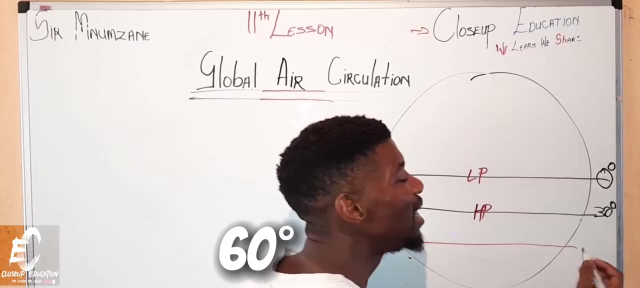 on a high pressure when we are on 30 degrees. okay, remember, the cold air is the one that it has now descended. so this cold air will obviously stay on earth until it converges with another air or it receives direct insulation from the sun, and it obviously happen when we reach our 60 degree mark. 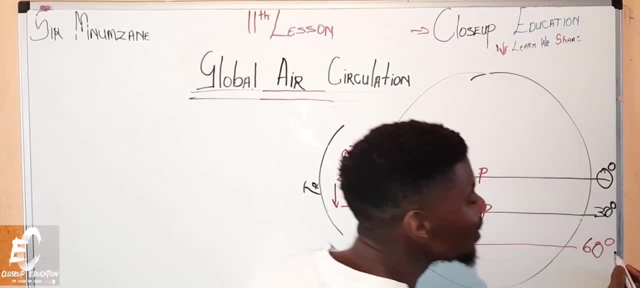 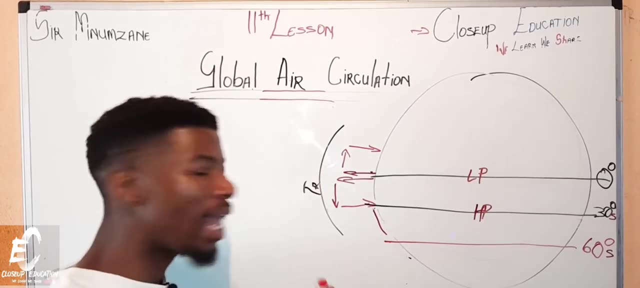 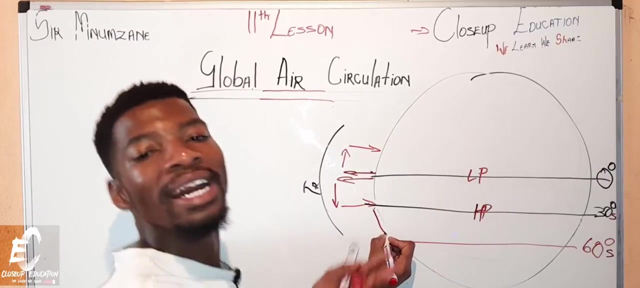 this is the 60 degree mark. remember, this is Southern Hemisphere- right, 30 degrees south, 60 degrees south. so now what we have here: when the air converges or when there's another insulation, this will obviously mean the air will rise again. the air is now rising right as the air. 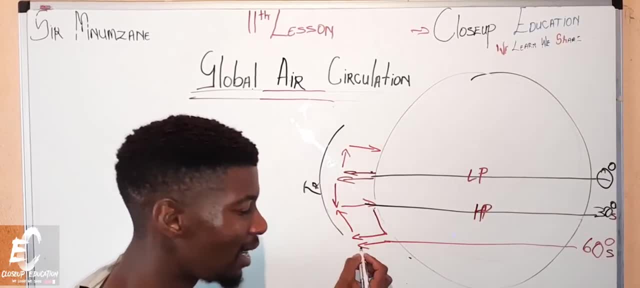 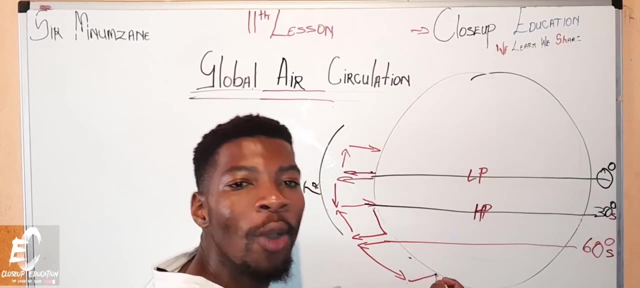 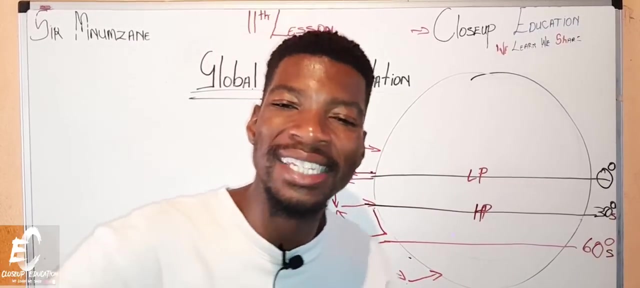 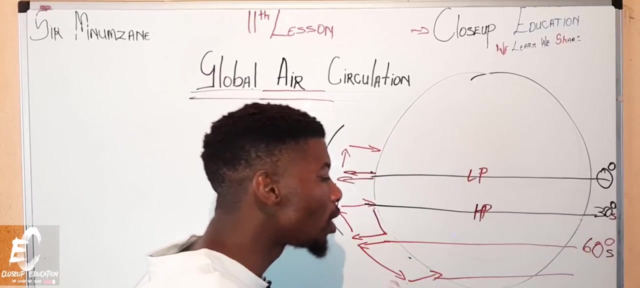 rises, it will obviously do what diverge: diverge, right as the air is diverging, it will obviously arrive to a point where it has to sink because of the higher you go, the colder it gets. so when it sinks it obviously cause there are what we call a high pressure, so it will cause what we call. 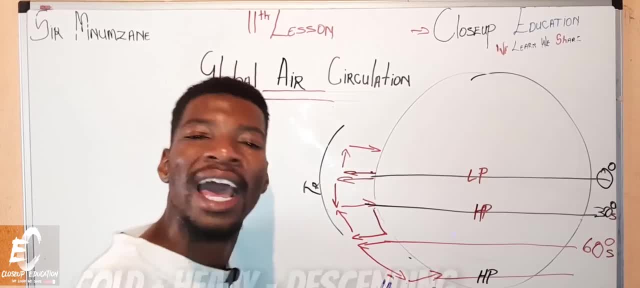 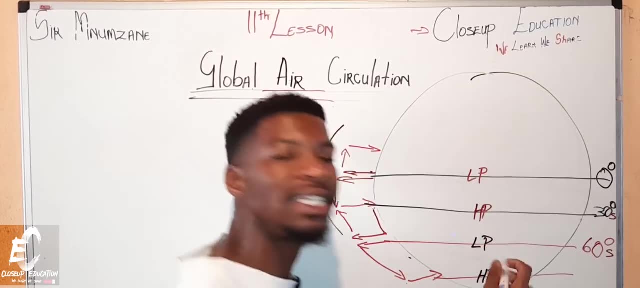 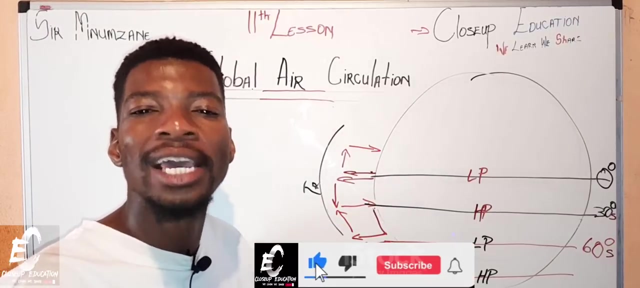 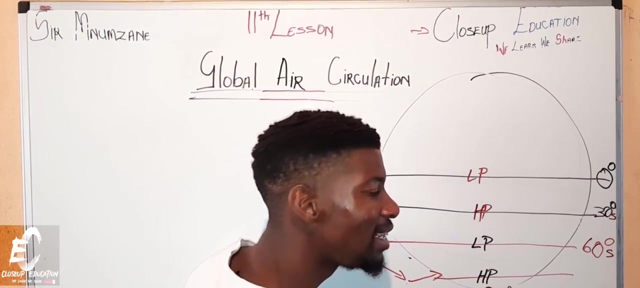 a high pressure because of now there is cold air descending towards earth, so there's a high pressure. now this is no pressure because of the air is ascending, all right, so now we know the air circulation. how is the air circulating around these latitudes? yes, and we write our 90 degrees south there. all right, remember what we have done down here it is: 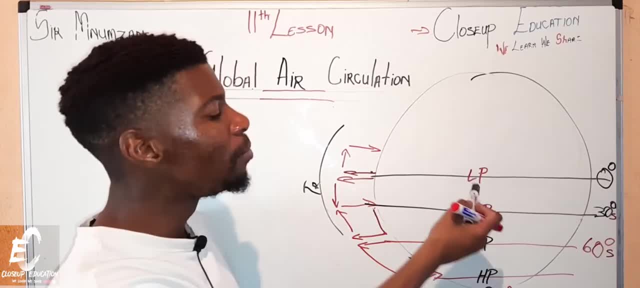 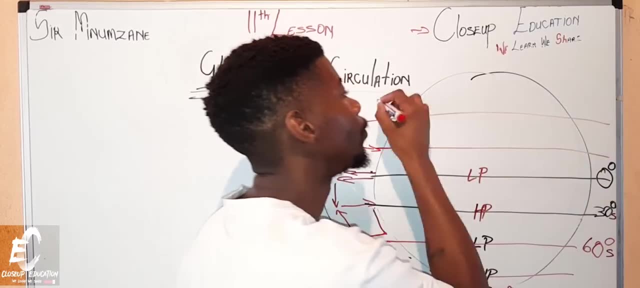 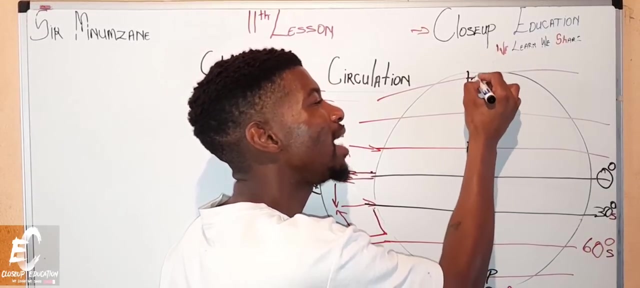 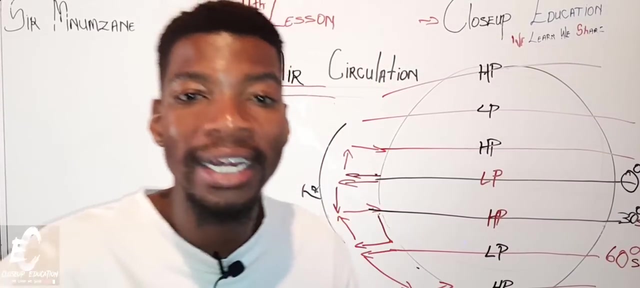 definitely the same up here. it will obviously mean there will be high pressure, low pressure. right, this is what we do. right, we know that there is high pressure, low pressure and high pressure. why does the cold areas consist of high pressure? because of we know that they do not receive direct insulation. 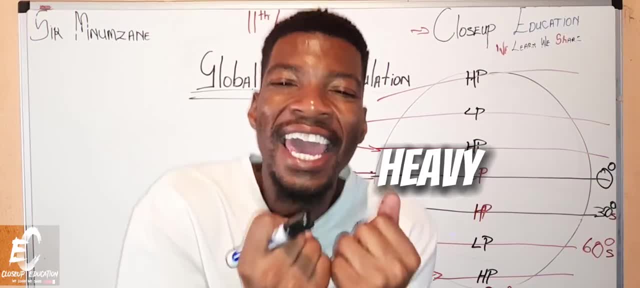 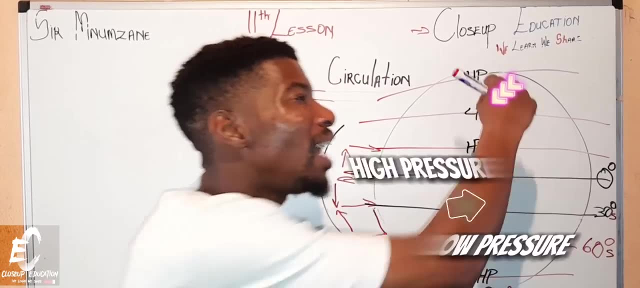 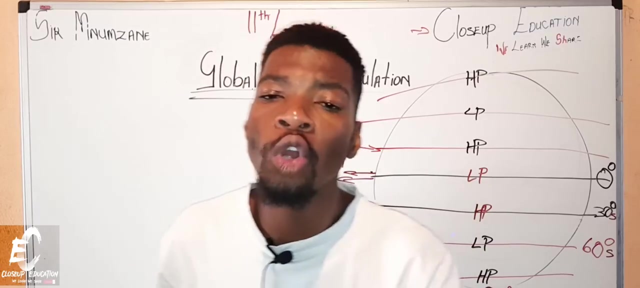 from the sun, meaning the air there. it is heavy, cold, dense, it is always sinking. all right, we know that air moves from high pressure to low pressure. right, we know that, that our air moves from high pressure to low pressure. if you do not know that, watch the video i dropped before this one, because 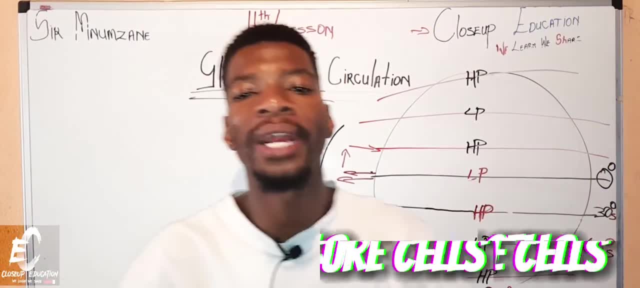 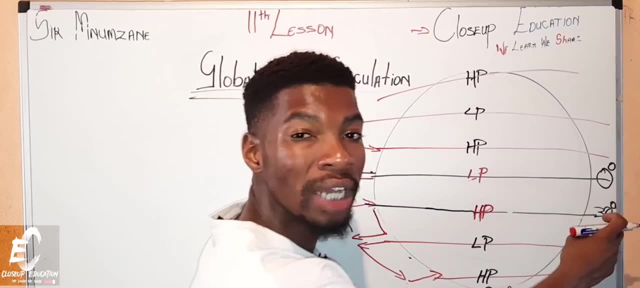 of. we are moving forward all right, now that we know the pressures within the earth, this will definitely mean we now have to understand the areas between 0 to 30, 30 to 60 and 60 to 90. all right, we know that there's zero. 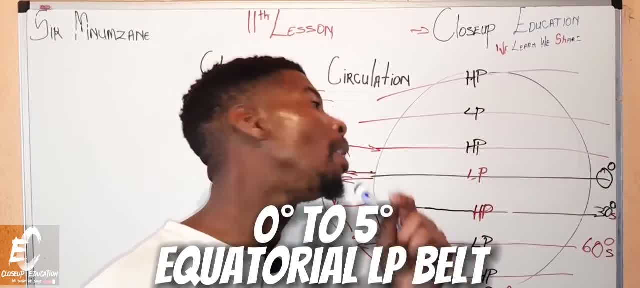 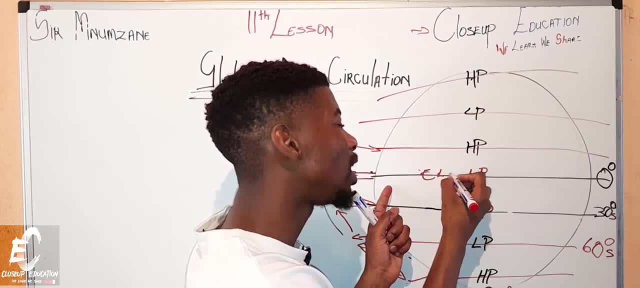 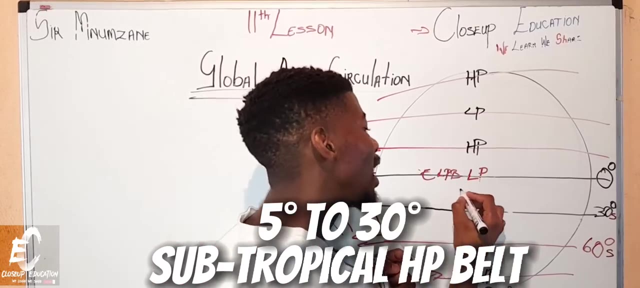 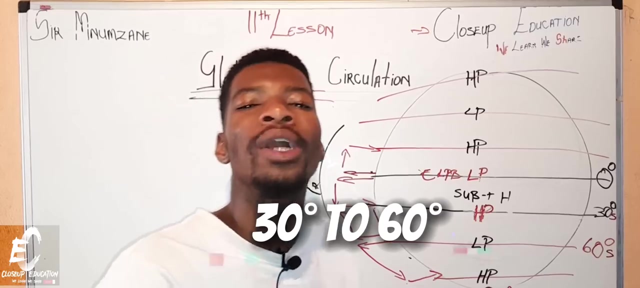 it is called the equatorial low pressure belt. right, this is our equatorial low pressure belt. i do not have a space here. low pressure belt, equatorial low pressure belt, and here we have our subtropical high pressure right, our subtropical high pressure right, and between 30 to 60 we have our 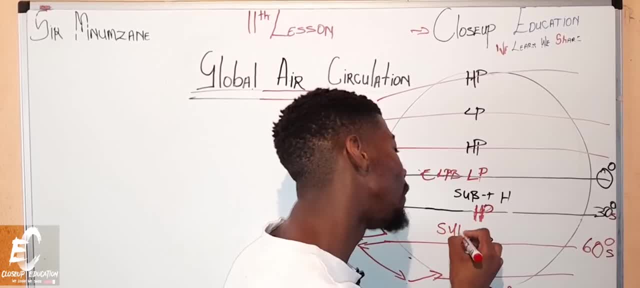 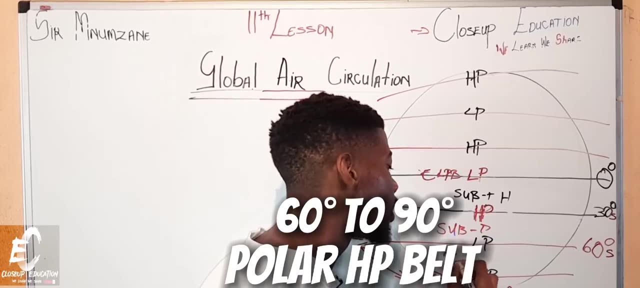 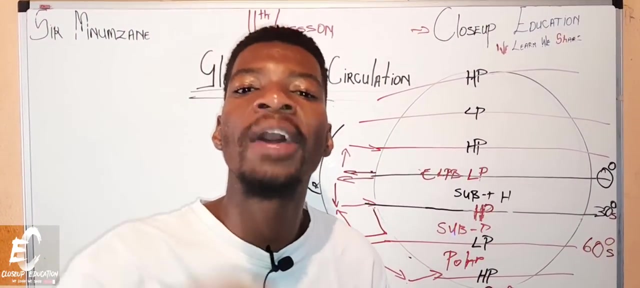 sub polar. yes, sub polar. this is our sub polar, and between 60 to 90 we have our polar. this is our polar high pressure belt. all right, and what do we call these things on the side? we gave them names. they have names. This is called a hardly sail. 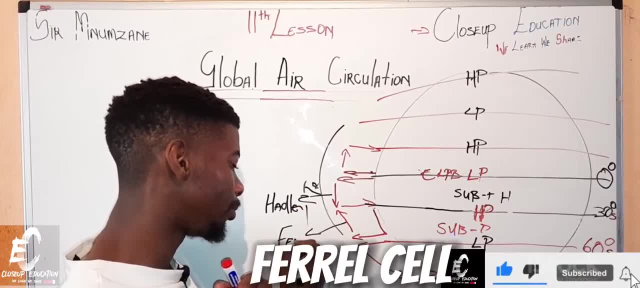 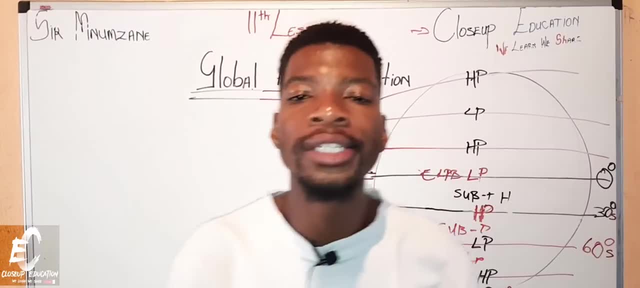 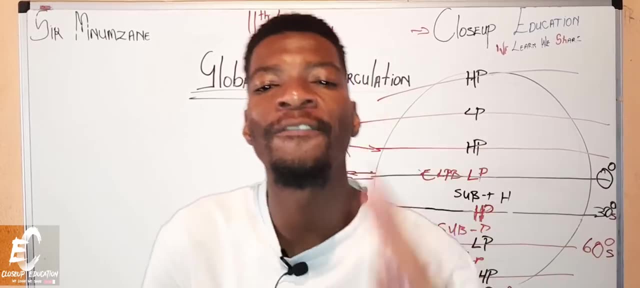 And this is called our Pharrell sail And this is called your homework. Get what this is called. Alright, let's continue. How does the wind move? This is the part we've been waiting for. The wind is pushed by the force which we call a Coriolis force. 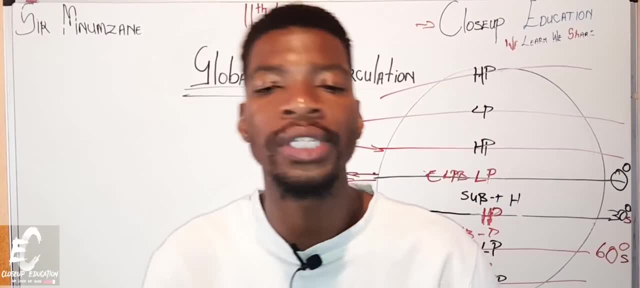 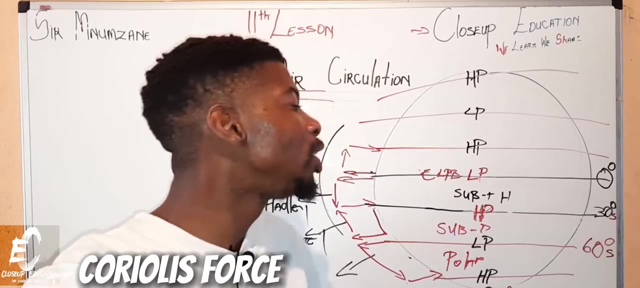 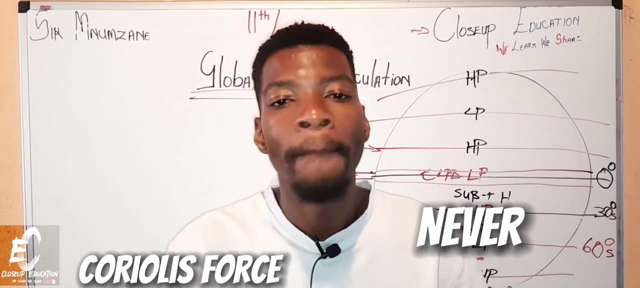 This force determines how the air has to move or rotate according to the rotation of the earth. We know that Coriolis force it is not strong between 0 to 5 degrees. Coriolis force can never be possible between 0 to 5 degrees. 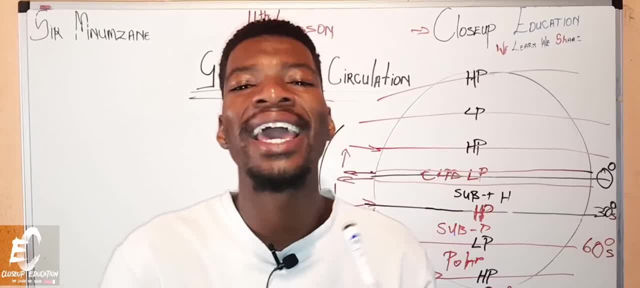 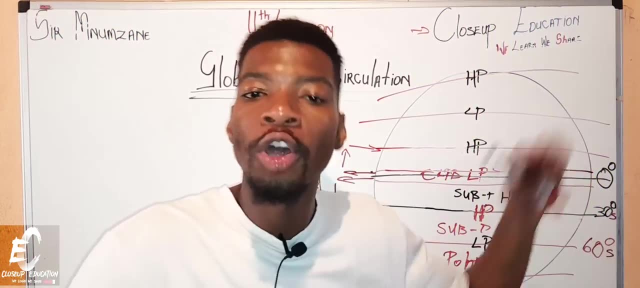 Meaning at the equator, at the center. there is less wind there. Alright, let's continue. Okay, From the 5 degree mark north or south, the Coriolis force starts to kick in And then it affects the movement of the wind. 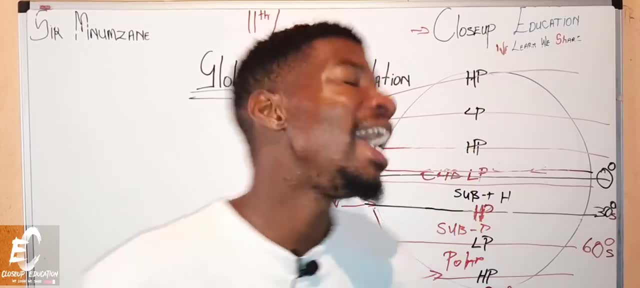 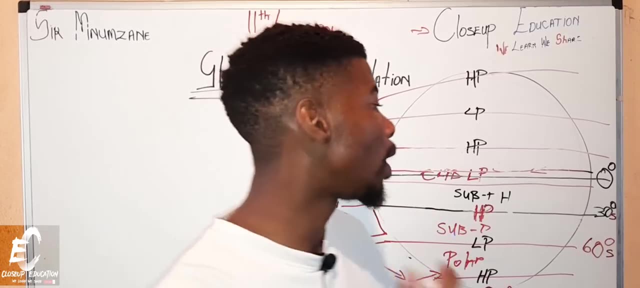 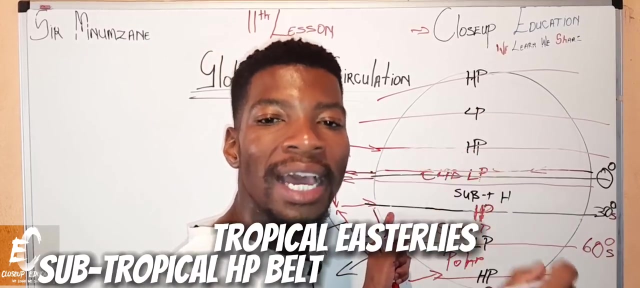 In the northern hemisphere, the wind will move to the left, And in the southern hemisphere, the wind will move to the right. Alright, let me draw it down so that you could understand. Alright, we know very well that in the subtropical high pressure we have tropical easterlies. 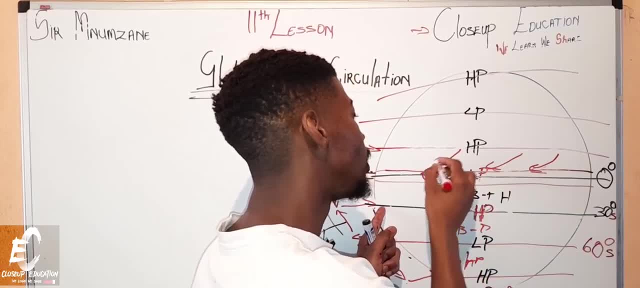 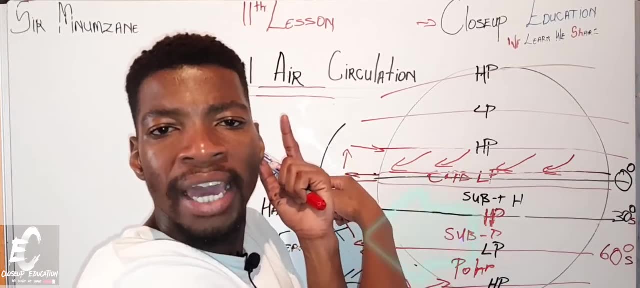 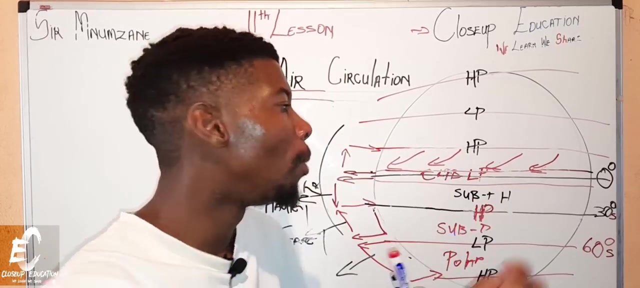 They look like this. Right, These are what we call tropical easterlies. Why tropical easterlies, when they look like they are looking or facing west? Because we name the wind according to where they are coming from. So they are coming from the east. 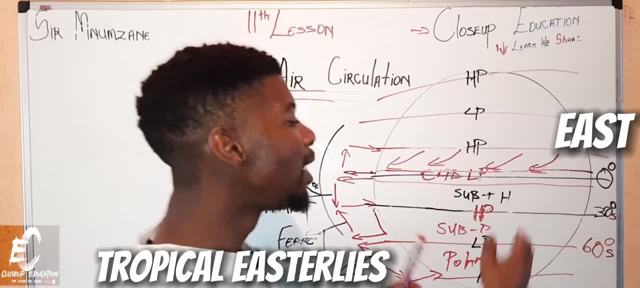 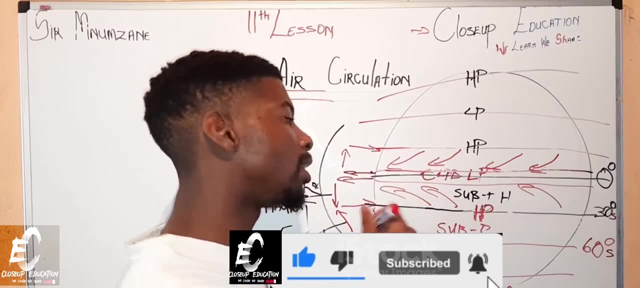 That's why we call them tropical easterlies, Meaning this side. it has to obviously look like this, It has to look like this, It has to look like this, Right? So these are the tropical easterlies, Alright. what about between 30 to 60?? 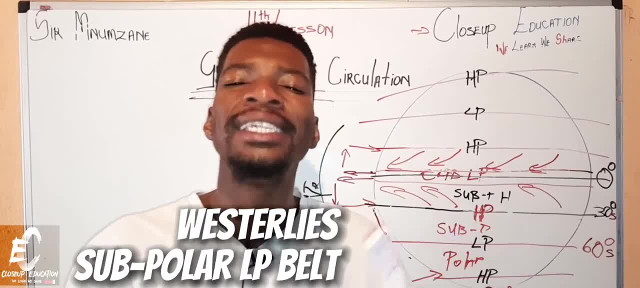 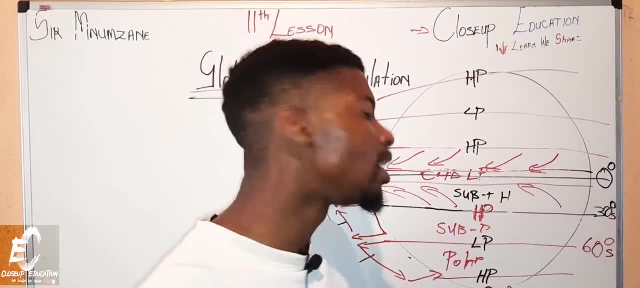 Which winds do we have there? We have westerlies, Yes, westerlies. This is where I stay, This is where South Africa is. We find westerlies. How do westerlies move? They move like this Right. 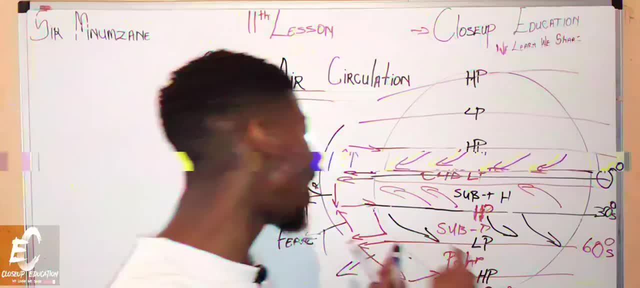 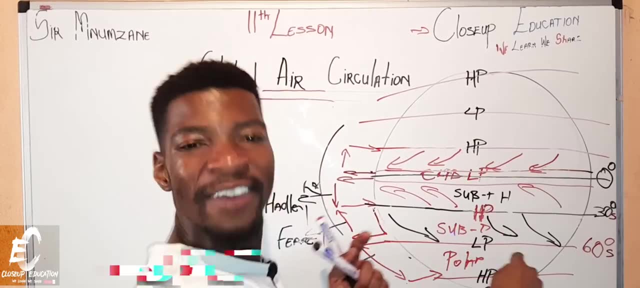 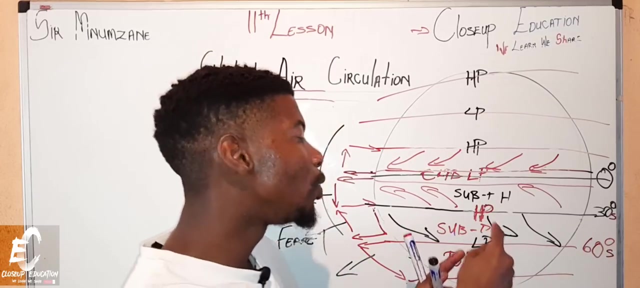 Like this. Right, They are moving from the west to the east. That's why they are called westerlies. And remember, why are they facing down? Because of Because of air pressure decreases or moves from high pressure to low pressure. 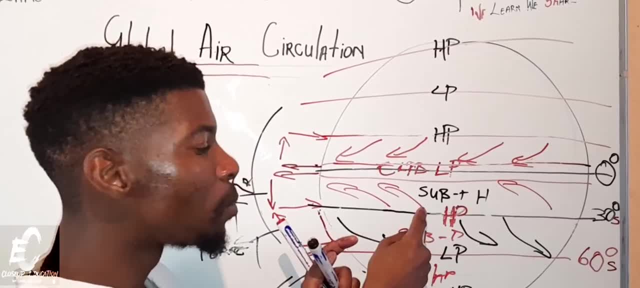 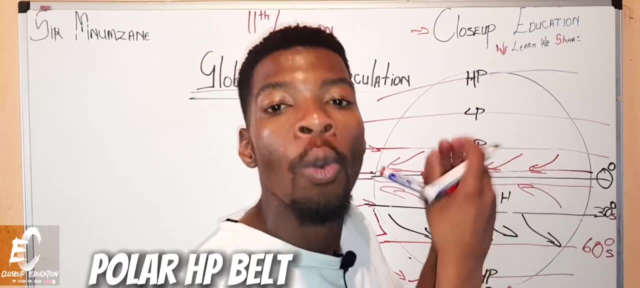 From high pressure to low pressure. That's why it's moving from high pressure to low pressure. where there is an equator, Right Then we are going down there. What is the wind which we'll be finding down there? It is what we call the polar easterlies.